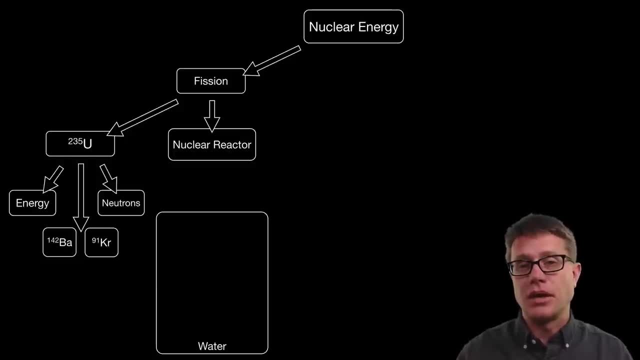 in a weapon. it is controlled in a reactor. Most of the reactors in play right now are light water reactors or normal water reactors. What you do is you put fuel rods inside And as the decay it produces a little bit of energy And that energy inside the water. 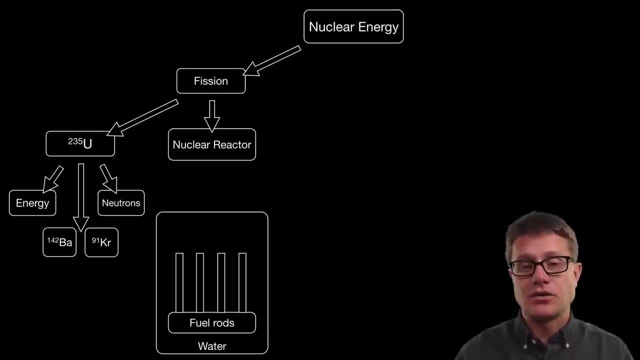 heats it up And we can use it to generate steam and then generate electricity. Now, when it melts down, this goes out of control And we get a release of that radiation into the environment, And so by having it in water, we can contain some of that energy And we 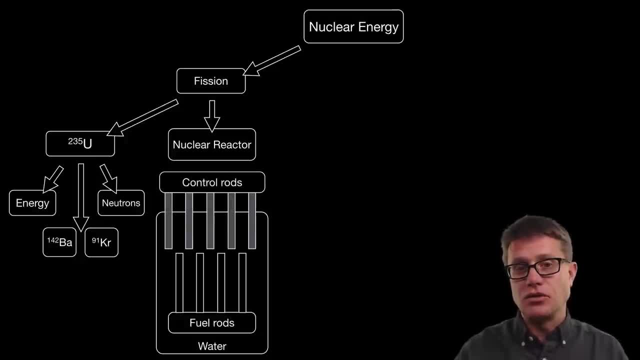 can also use control rods. These are actually going to take in some of those neutrons And by lowering them between the fuel rods we can slow down the reactor. Now the disadvantages are pretty apparent: Nuclear waste is going to be created, And it can be around for thousands. 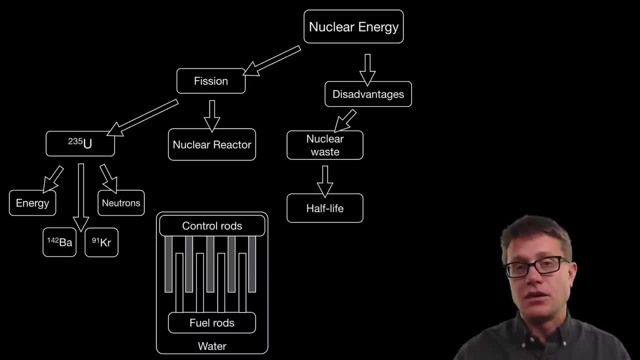 and thousands of years. So we have to keep track of that. Each of the radioactive materials have a different half life, But it is going to be on the order of thousands of years And also we have these accidents, where we can have explosions, malfunctions and it releases. 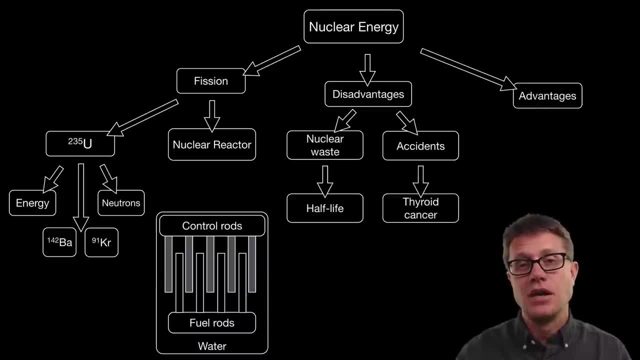 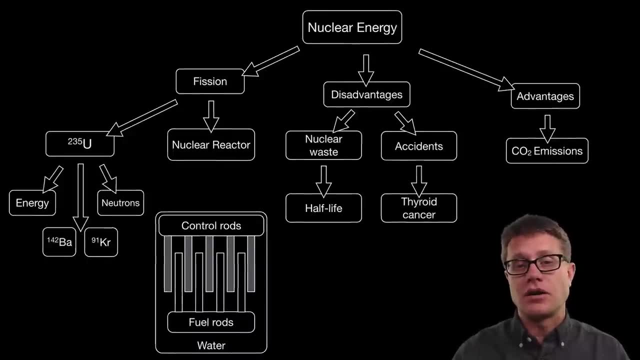 that radiation into the environment and can cause things like thyroid cancer. Why do we still have it? Well, the advantage is that it creates a huge amount of energy, and it can do that without increasing the amount of carbon emissions in the environment. So if we look at uranium-235, now we are looking just at the nucleus And so we are looking. 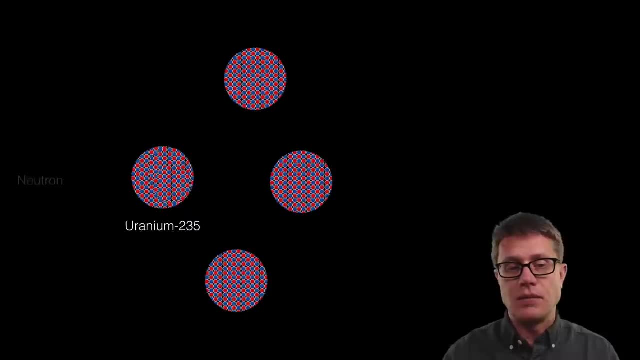 at the protons and the neutrons. And so if we were to hit one of those uranium atoms with a neutron, what it will do is it will break in half, It breaks apart into these two fragments And as it does that, it releases a certain amount of energy. You can see it. 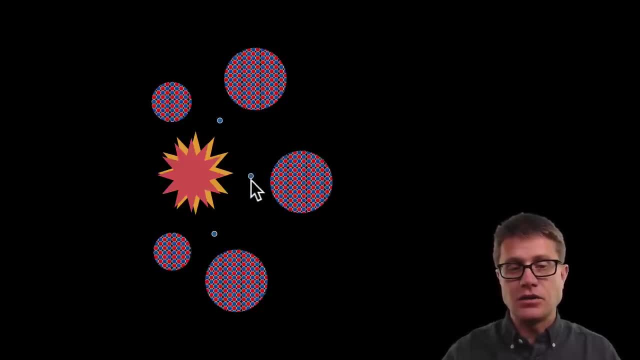 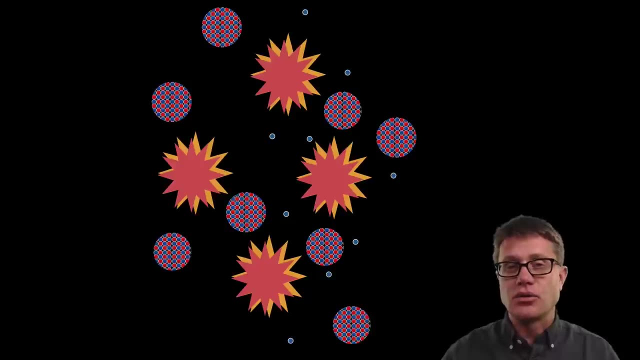 is also liberating three of these neutrons, And each of those have the potential to hit another uranium-235 and we can break it down. So it is not an out of control chain reaction like this that we might want to do, But it is a very powerful reaction And it is a very 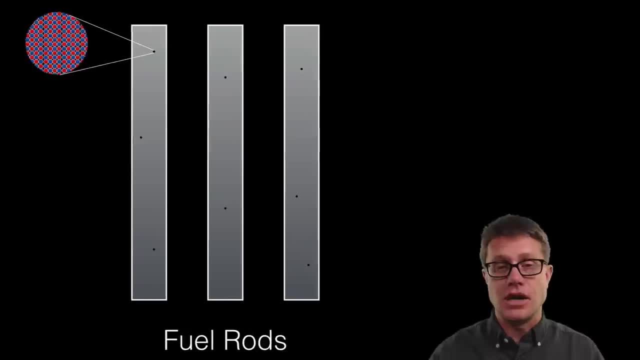 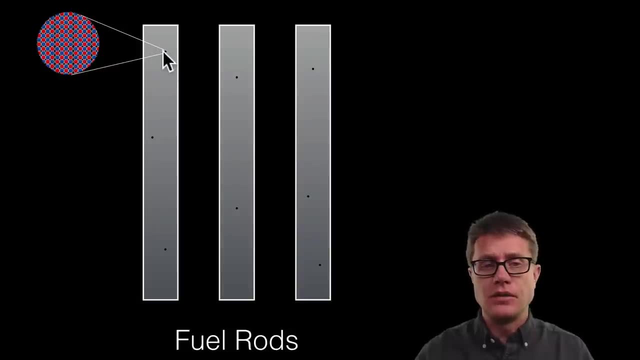 powerful reaction that we might see in a nuclear bomb, But it goes slow over time. And so, if we look at what those fuel rods are like, most of the uranium is actually going to be uranium-238.. A few of it is uranium-235.. And so, as those neutrons are given off by 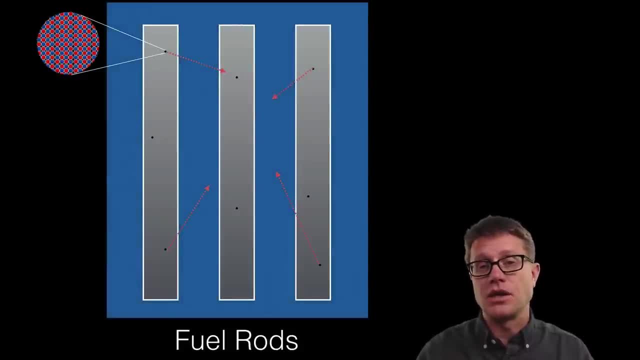 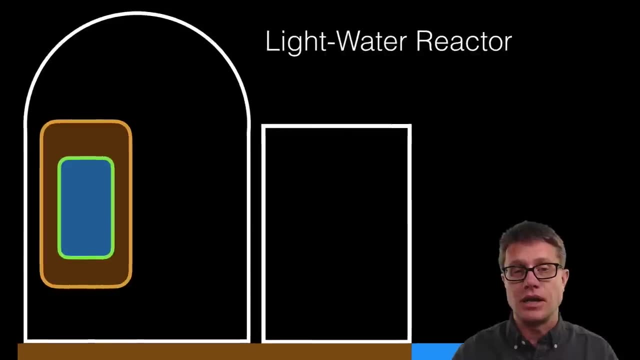 having it in water, we can absorb some of that energy and we can control that radiation. And also we can lower these control rods. They absorb the neutrons and so we can slow it down. So if we look at a typical light water reactor, we are going to have the fuel. 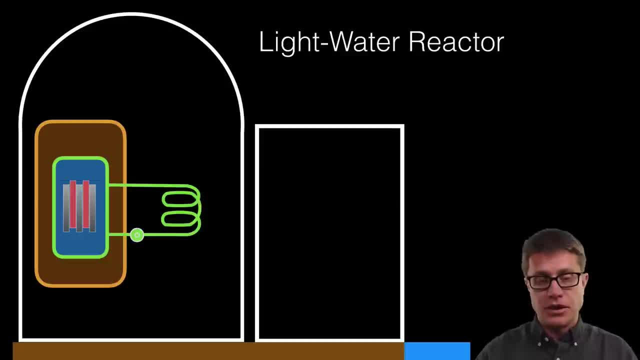 rods and the control rods in the core. We are then going to heat up a fluid, And that fluid is going to be in a closed system, So as it moves through these pipes it returns back where it was, But it is bringing with it a huge amount of heat. Now that heat moves, 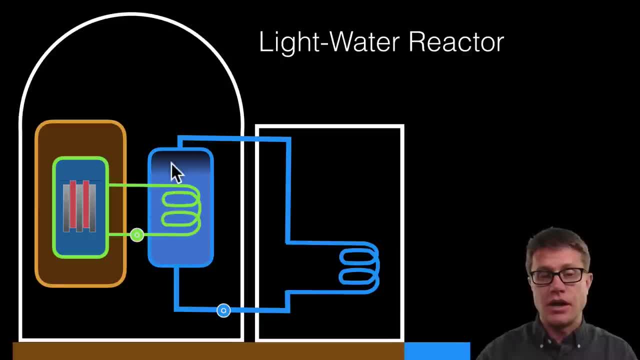 into a separate loop, And so in this loop what we are doing is we are heating up the water, It is forming steam up at the top, And then that steam is moving through a generator, So we are generating electricity And then, finally, we still have a lot of heat, right. 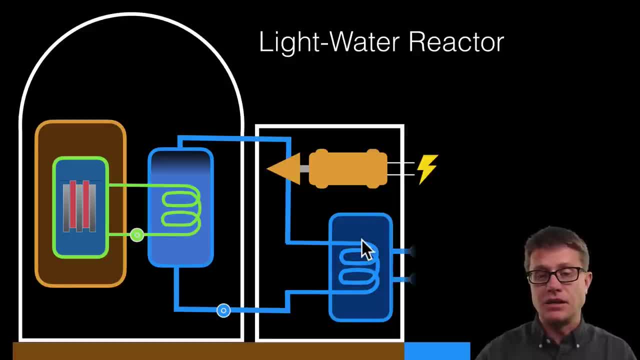 here. But so before we pump it back in, we have to get rid of some of that heat, And so we are going to do that by pumping the water and another loop into a cooling pond, And so, as long as we have energy contained within those fuel rods, we can generate electricity. 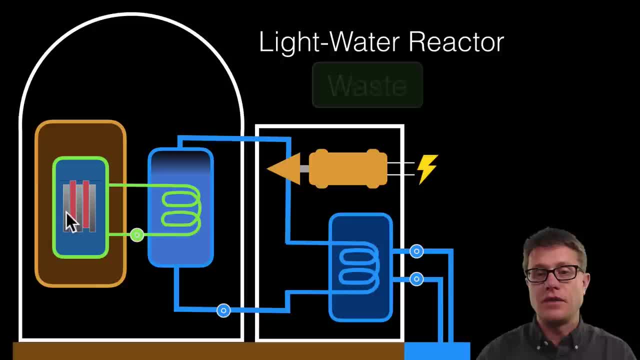 But what happens when we decay too much of that uranium-235?? Now it becomes waste. It is still radioactive, but it is not generating enough electricity for the plant to go, And so now we have generated waste. So that is one form of nuclear waste, But we are also 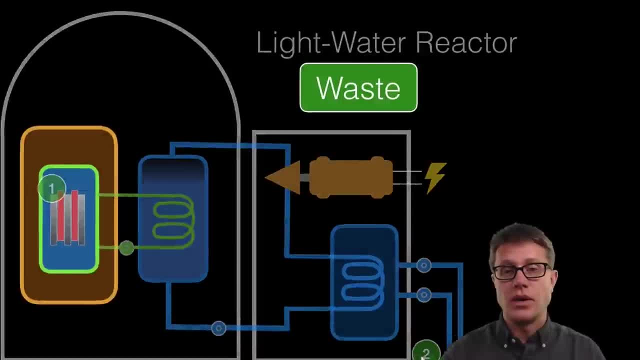 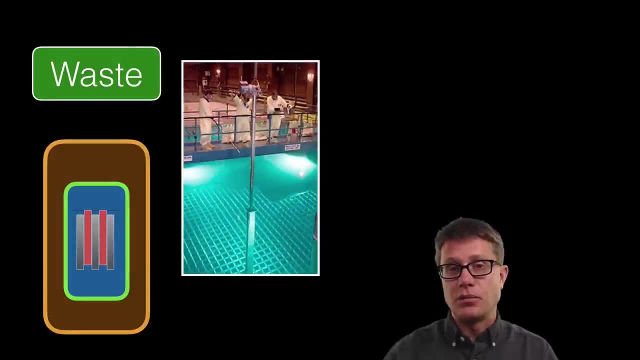 generating a little bit of heat over here into the environment as well. So we are going to have to deal with that waste. And so how do we deal with that waste? Well, how do we deal with those fuel rods? We are going to put them in a pool And, as we put them in, 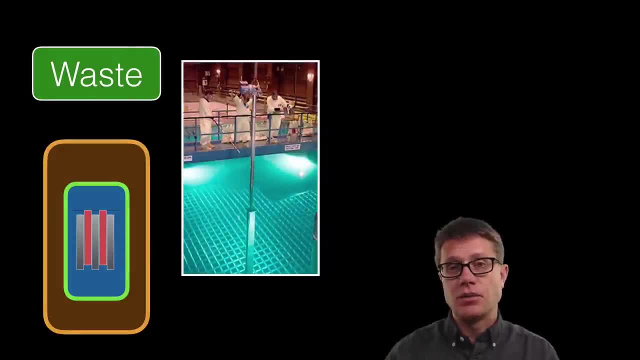 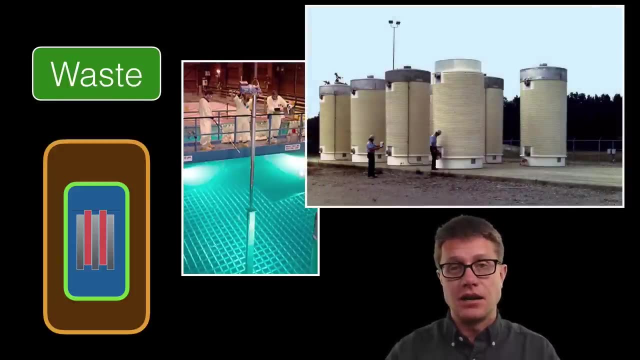 a pool. we are going to absorb some of that energy here, But eventually we are going to have to put it in some kind of a container And a lot of these are on these concrete slabs And we have got that nuclear waste contained inside there. There is no real long range. 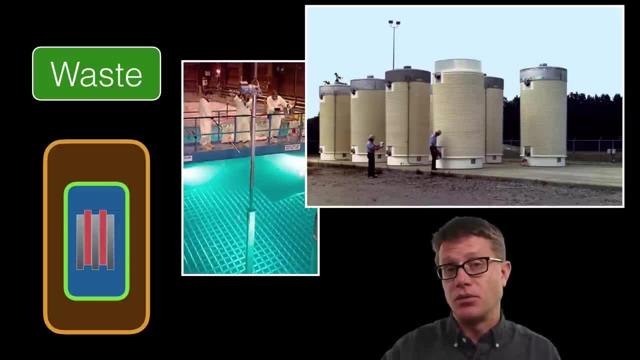 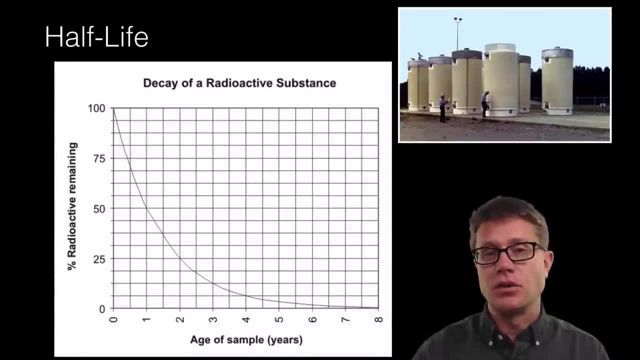 plan of what we are going to do with this nuclear waste And it is going to be a problem that we will have to deal with generations down the line. If we look at how long this could occur, you have to understand what a half-life is. A half-life is going to be a. 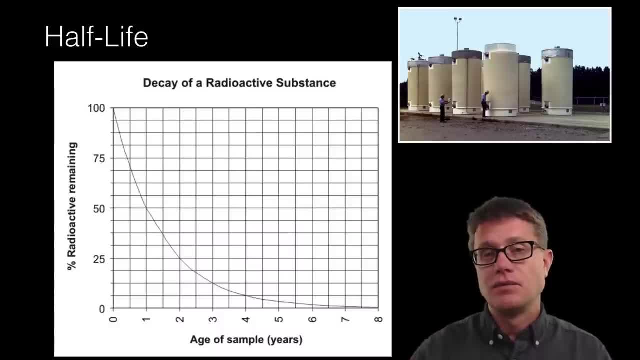 the amount of time it takes for half of the material to decay or to break apart. And so if we look at time 0, let's say the half-life is one year- At time 0 we would have 100% of the radioactive material. At time 1 we would have 50% of it, In other words, half of it. 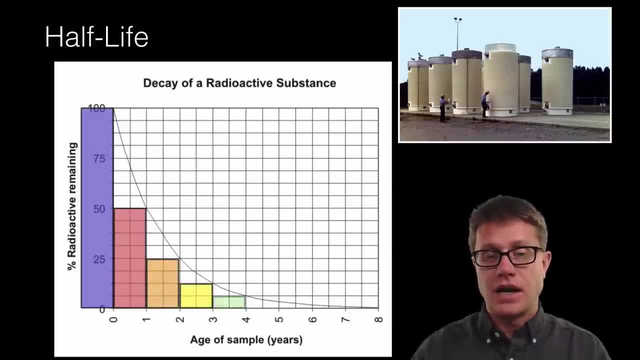 would have decayed In another year. it would be half of that and a half of that and a half of that and a half of that. And so in an AP environmental science class you should life. And let me give you a problem. Let's say radium has a half life of 1500 years. 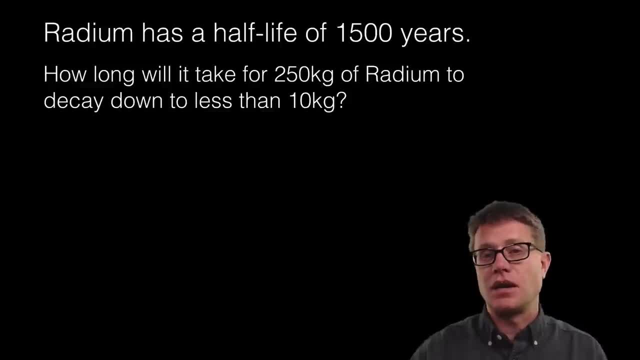 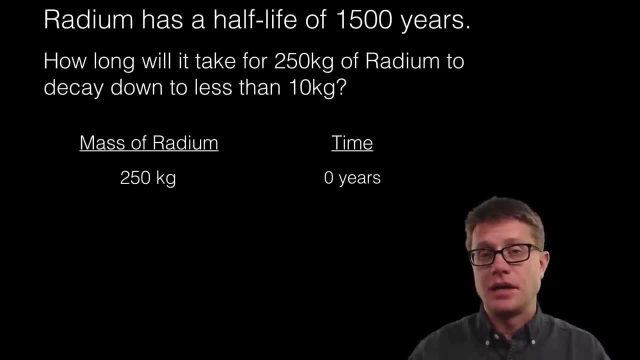 How long will it take for 250 kilograms of the radium to decay down to less than 10 kilograms? And so we are saying the mass of radium at the beginning is 250 kilograms at time 0. And so in one half life, in other words in 1500 years, we would have decayed half of 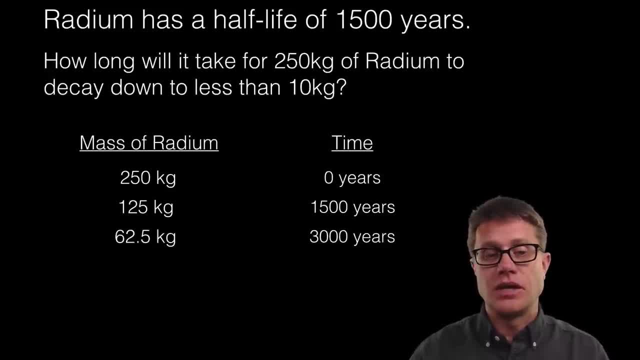 it down to 125.. In another 1500 years we would be down to 62.5.. And you can just keep doing this. and you can see, at 7500 years we are less than 10 kilograms left, But you can see. 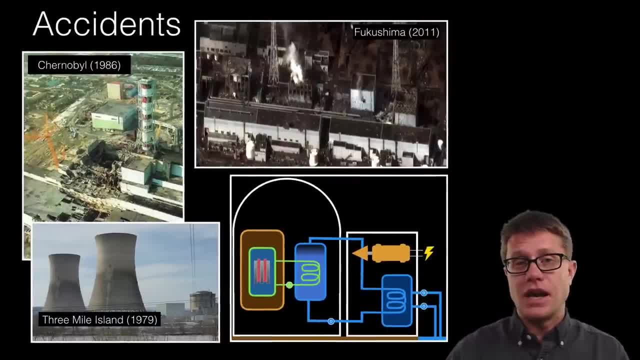 a lot of that is still going to be radioactive. Now, what happens in accidents? Something happens where we are not able to contain this core. And so, if we look at Chernobyl, they were testing the reactor and it got out of control. It heated. We have a melting or an explosion. 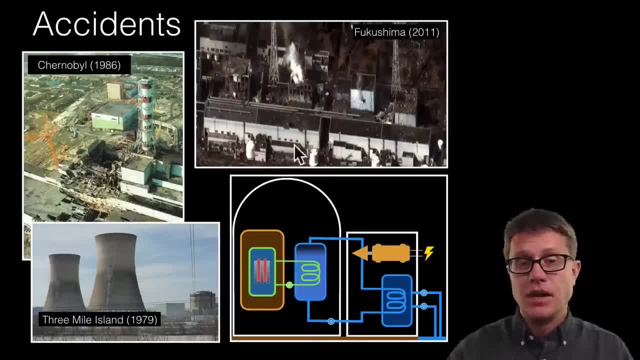 that actually collapsed the roof. It released a lot of radiation. If we are looking at Fukushima, it is like three levels of protection that failed. We have an earthquake, We have a nuclear mistake, But we also have this giant tsunami. And if we are looking at Three Mile Island, 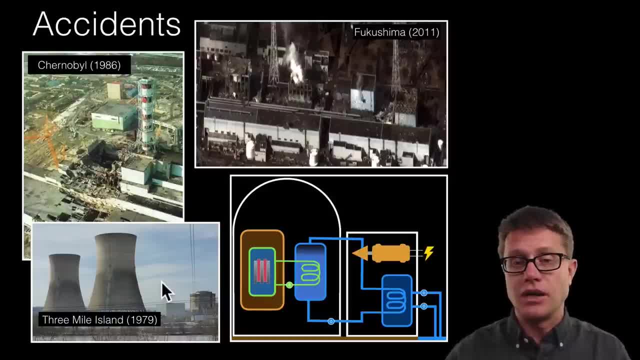 it was a problem with a valve, but also a problem with user error as well, And so all of these, for the most part, are human error. Either we had a mistake at the reactor or had a mistake in the design, And what it does is it releases some of this radioactive material into the 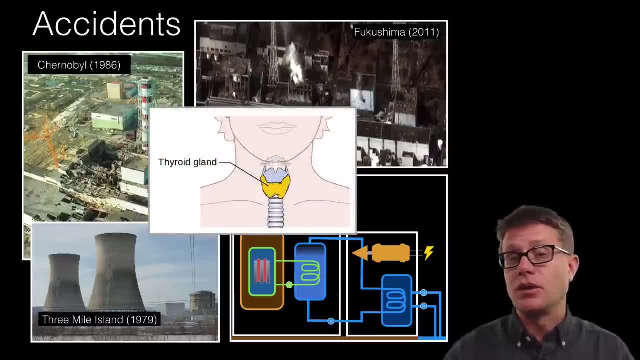 environment. So, for example, radioactive iodine can cause thyroid cancer, So we eat it in our food. It causes cancer years down the line And we are going to see this wherever there is a nuclear accident. We are going to have increases in thyroid cancer after that. So if we look at these, 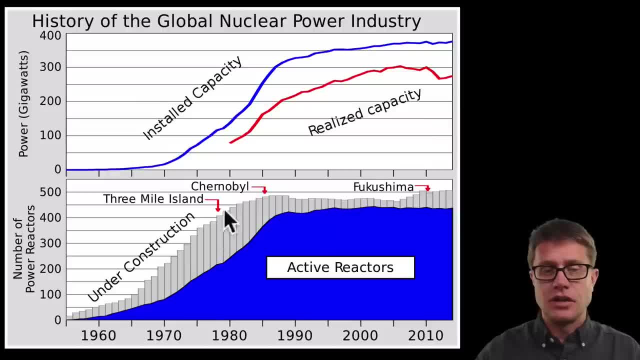 accidents. so this is it. Here is Three Mile Island, Here is Chernobyl. So we had the heyday of nuclear reactor creation during this oil crisis, But then, after these accidents, you can see the amount of reactors that we have has remained static, And you can say even: